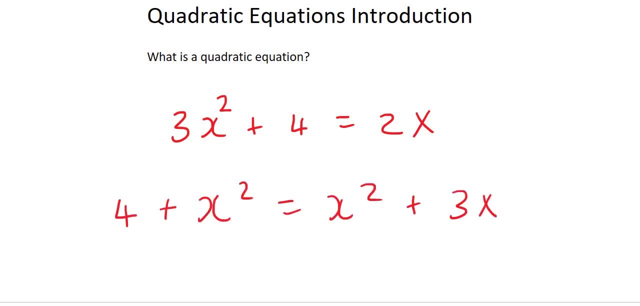 it actually is not. Let me show you an example. What would happen here if we have to take, for example, this x squared and we add an x to the power of 2, then all of a sudden it is called a quadratic equation. Now, if I add an x squared over to the left hand side, is that you would end up? 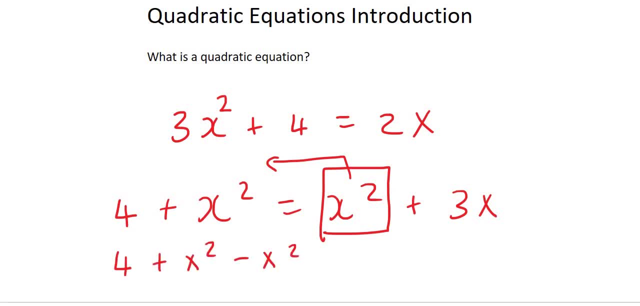 with something like 4 plus x squared, minus x squared equals to 3x, and these x squares would cancel out. So what looked like a quadratic equation in the beginning actually turned out to be a normal equation. So we will only say that it is a quadratic equation if there is an x squared. 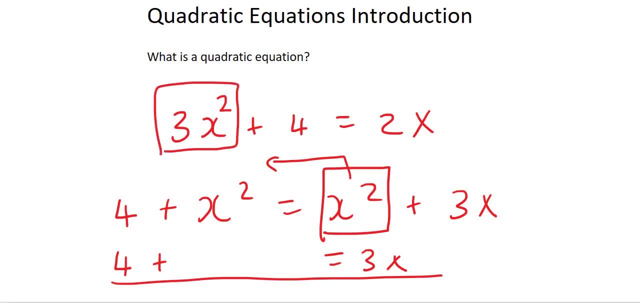 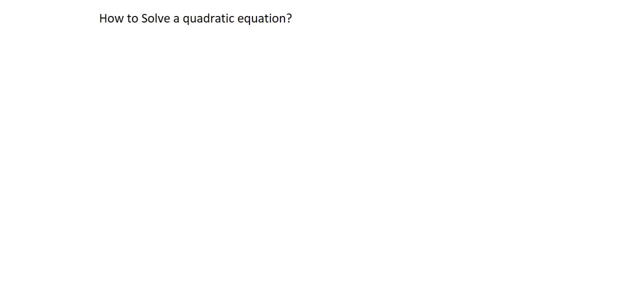 that does not cancel out with another x squared. Here is another example. I am now going to show you how to solve a quadratic equation. So what you do? let's say we have an example like this, Alright, so there we have a quadratic equation because it's got that x squared. 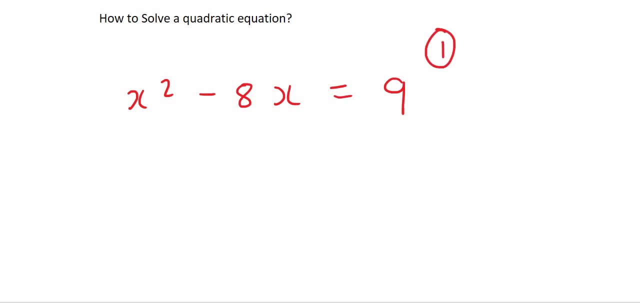 that we spoke about. Step 1, move everything to one side. So, for example, this 9, we are going to move over to the left, so it's going to become x squared minus 8x minus 9 equals to 0.. When you 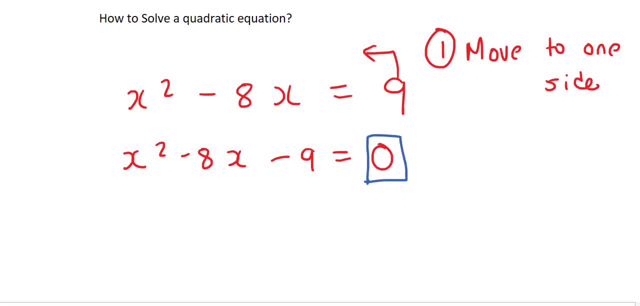 see the 0. that's a good thing. You want the 0 on the left or the right, It doesn't really matter, but you do want that 0.. Once you have the 0, then you're going to factorize. Now there are many different ways that you could. 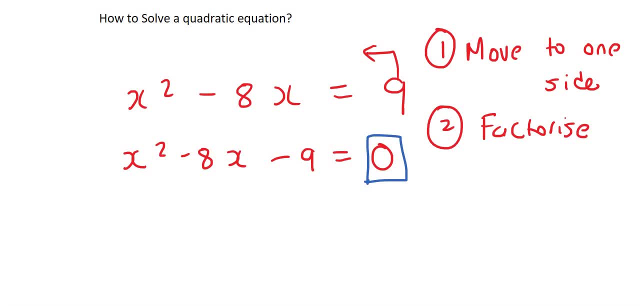 be asked to factorize. We know that there is difference of squares, common factors, trinomials, So look out to see which type of factorizing you need to do. If you're quite good with your factorizing, you would know that this over here is a trinomial, So we would have to factorize it as 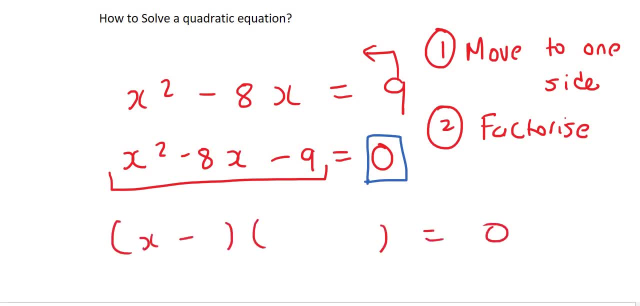 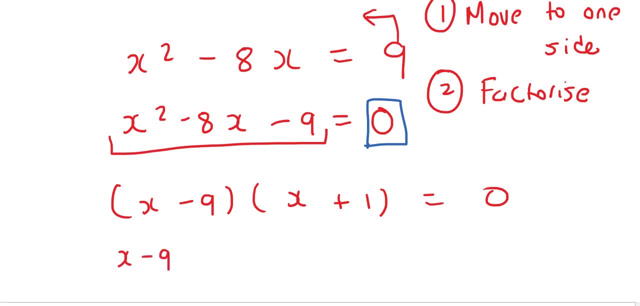 a trinomial. So we'll have two brackets and it would be x minus 9 and x plus 1.. What you now do, when you've got these brackets, is you say x minus 9 must be equal to 0, or x plus 1 must be equal to 0, and then you 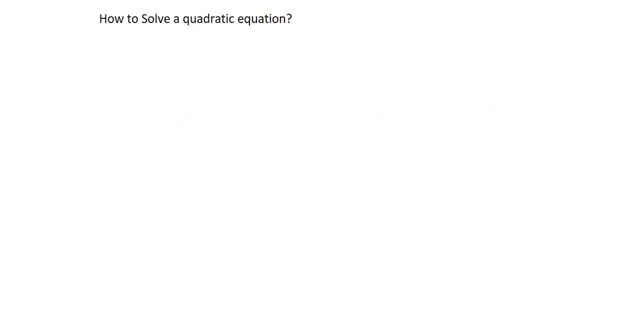 I am now going to show you how to solve a quadratic equation. So what you do, let's say we have an example like this. Alright so there we have a quadratic equation because it's got that x squared that we spoke about. Step 1, move everything to one side. So for example this 9 we are going to move over to the left so it's going to become x squared minus 8x minus 9 equals to 0. When you see the 0 that's a good thing. You want the 0 on the left or the right. It doesn't really matter but you do want that 0. Once you have the 0 then you're going to factorize. Now there are many different ways that you could be asked to factorize. We know that there is difference of squares, common factors, trinomials. So look out to see which type of factorizing you need to do. If you're quite good with your factorizing you would know that this over here is a trinomial. So we would have to factorize it as a trinomial. 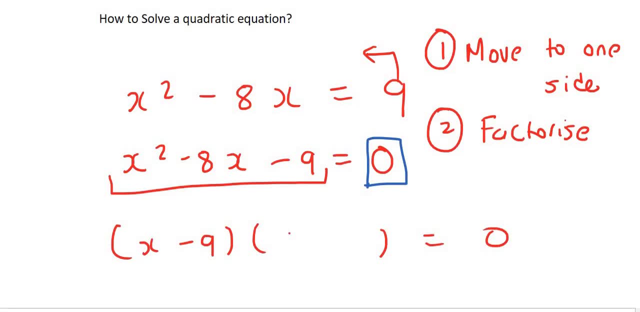 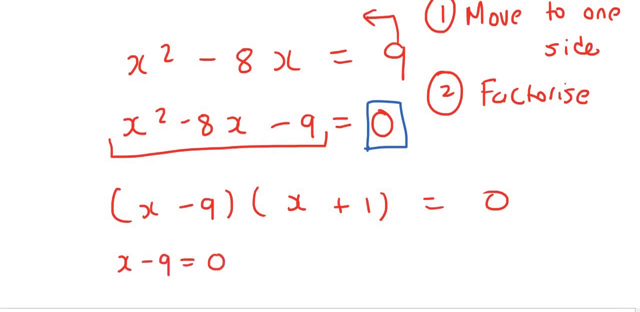 So we'll have two brackets and it would be x minus 9 and x plus 1. What you now do when you've got these brackets is you say x minus 9 must be equal to 0 or x plus 1 must be equal to 0 and then you go and you solve each of those. So this one here would be that x equals to 9 or and this one would say that x is equal to minus 1. Now we are going to have a look at four examples. For the first 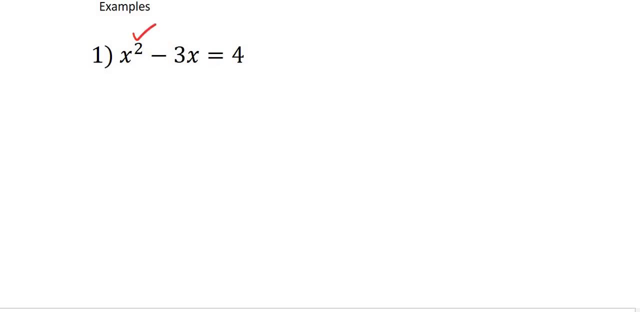 example we know that it's quadratic because it's got that x squared and it's not going to cancel out. So remember step one get everything to one side. So I'm going to say x squared minus 3x. I'm going to bring the 4 over. There we go. Now I've got the 0. The 0 is good. What we now do is we factorize. This is a trinomial. So it's going to be x minus 4 and x plus 1. I then say x minus 4 is equal to 0 or x plus 1 is equal to 0. So I'm going to say x minus 4 is equal to 0. So I'm going to x minus 4 is equal to 0. This then gives me x is equal to 4 or x is equal to negative 1. Here's 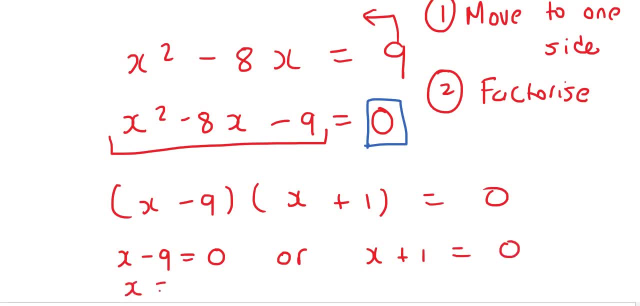 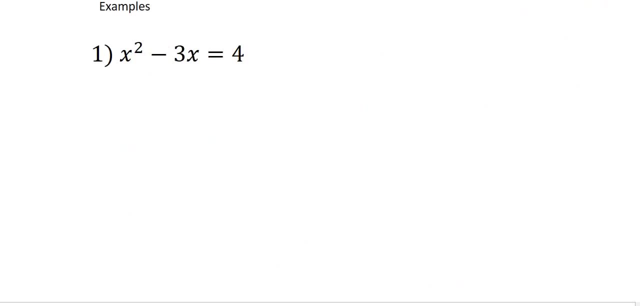 go and you solve each of those. So this one here would be that x equals to 9, or and this one would say that x is equal to minus 1.. Now we are going to have a look at four examples. For the first example, we know that it's quadratic because it's got that x squared and it's not going to cancel. 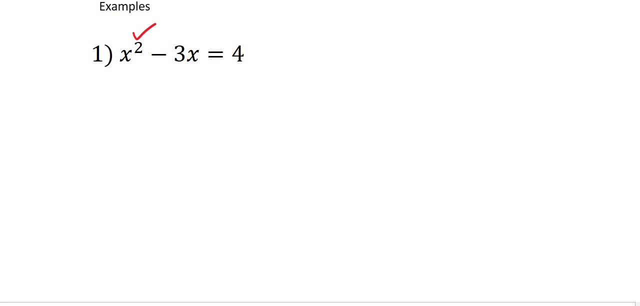 out. So remember step one, get everything to one side. So I'm going to say x squared minus 3x. I'm going to bring the 4 over. There we go. Now I've got the 0.. The 0 is good. What we now do is we. 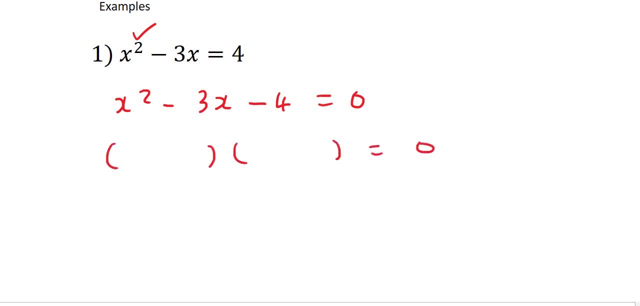 factorize. This is a trinomial. So it's going to be x minus 4 and x plus 1.. I then say x minus 4 is equal to 0, or x plus 1 is equal to 0. So I'm going to say x minus 4 is equal to 0. So I'm going to 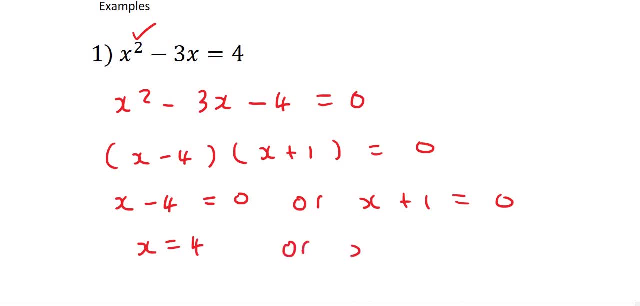 x minus 4 is equal to 0. This then gives me: x is equal to 4 or x is equal to negative 1.. Here's number two. We already have the 0, so that's step one complete. Now we factorize, Remember it's not. 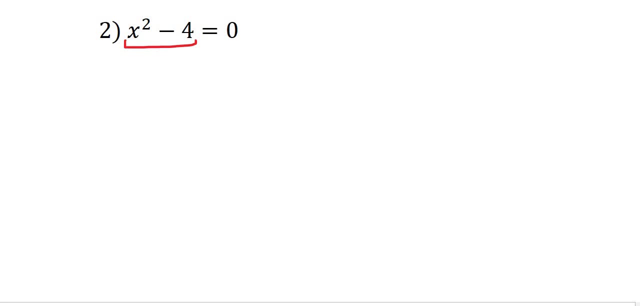 always going to be a trinomial. This is actually a difference of squares. So we open up two brackets where it'll be x minus 2 and x plus 2.. Remember that's how difference of squares work. and so we end up with x is equal to 2 or x is equal to. 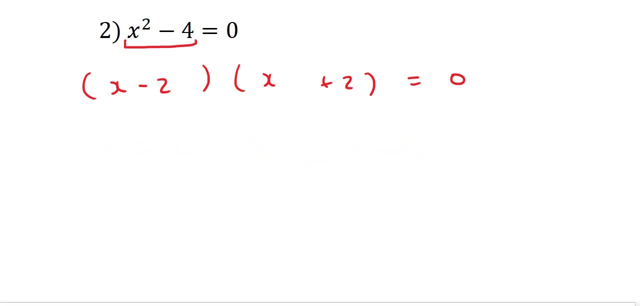 Negative 2. Actually I skipped a step there. I do apologize. I should say to be more or the more structured approach is to say x minus 2 is equal to 0, or x plus 2 is equal to 0. You then see that. 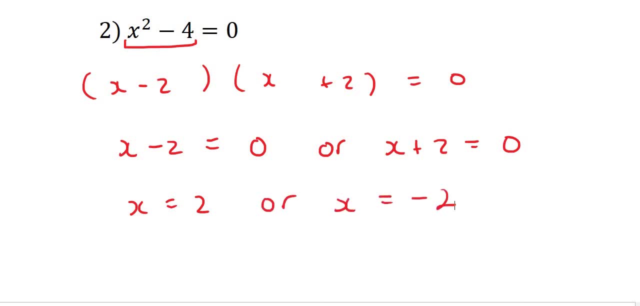 x is equal to 2 or x is equal to negative 2.. In question three we've already got the 0. So then we can factorize This over. here is a trinomial. So we open up our two brackets and we get x minus. 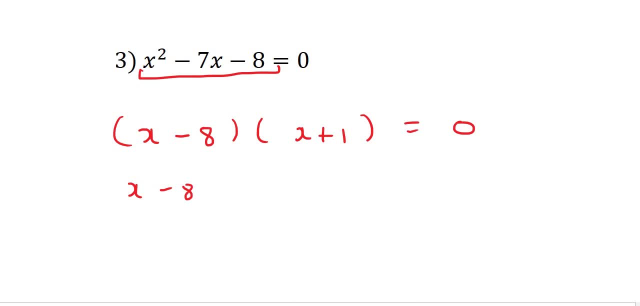 8, x plus 1.. We then say: x minus 2 is equal to 0. So we open up our two brackets and we get: x minus 8 is equal to 0 or x plus 1 is equal to 0. This then means that x is equal to 8 or x is equal to.